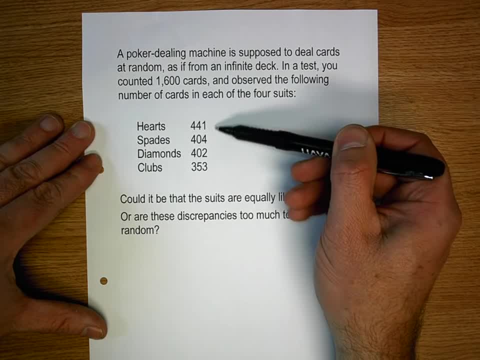 we want to be able to test to see if there's a significant difference between these observed values that you see here and the values that we've observed. So let's take a look at a chi-squared test and see if there's any values that we would expect in an experiment like this. Now, 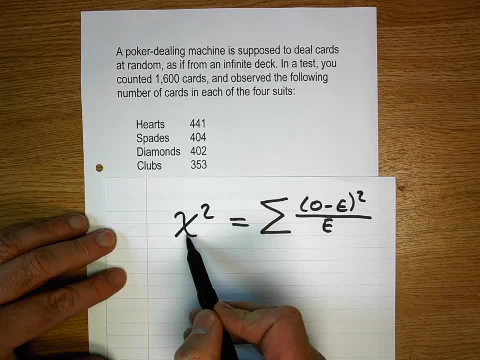 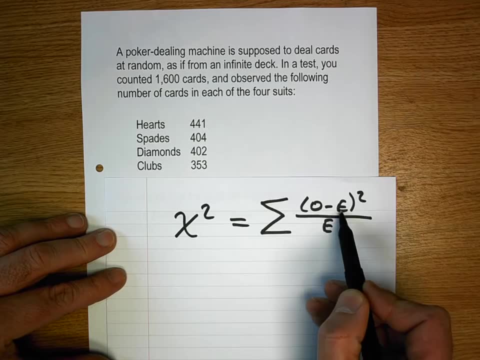 the formula that we're going to use for chi-squared is as follows. So this is my symbol here: chi-squared, It's equal to the sum of our observed difference between our observed and expected values: O minus E in here, squared divided by E, our expected values. So, as you, 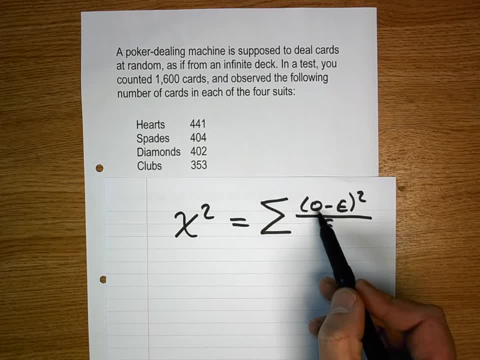 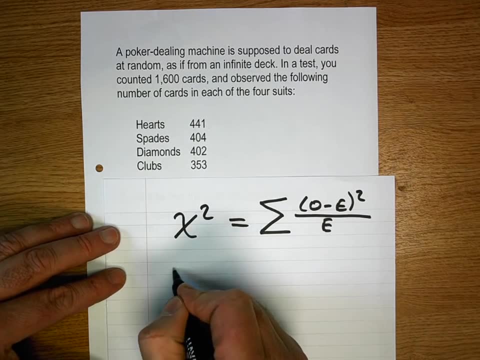 can see, we need just two values to help us determine chi-squared: O for observed, which we get from these values up here, and E for expected, which we will determine in a moment. So, before we start, let's outline our null and alternative hypothesis. Our null hypothesis. 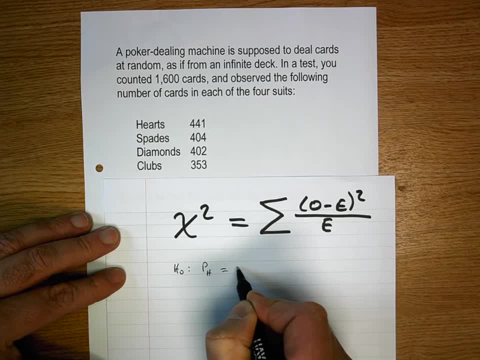 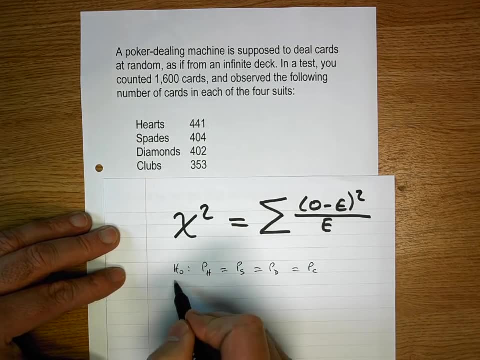 is that the proportion of hearts- H for hearts- is equal to the proportion of spades, is equal to the proportion of diamonds, is equal to the proportion of clubs. My alternative hypothesis is that they are not the same. So just putting in the not equals sign here And in a chi-squared. 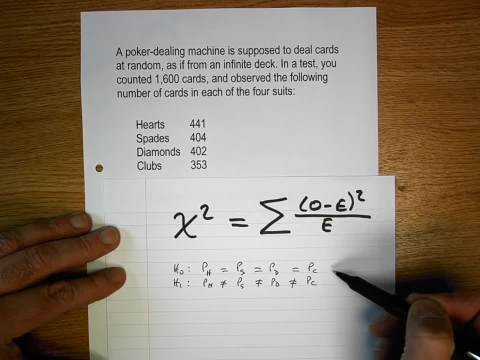 test, our null hypothesis test, tells us that there is no difference, no difference between the observed and expected values, And our alternative hypothesis is that there is a difference. so at least one or two of those are going to be different, And we're going. 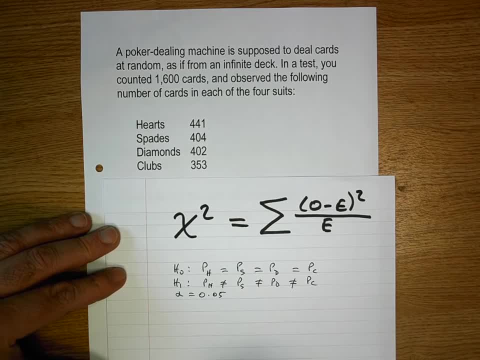 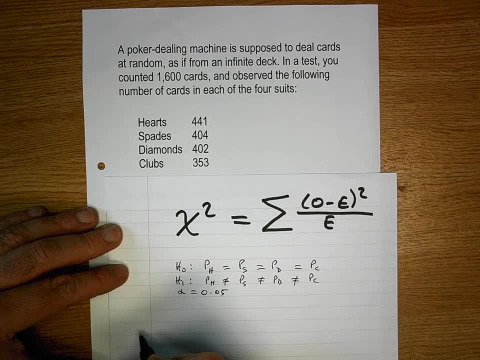 to operate here at an alpha value equal to 0.05.. So we're now ready to go and start to build up these values here, and I'm going to do this in a table. So first of all let me put down my observed values. So O for observed. so write in my hearts spades, diamonds and 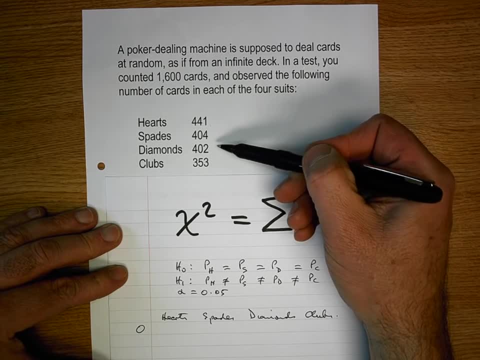 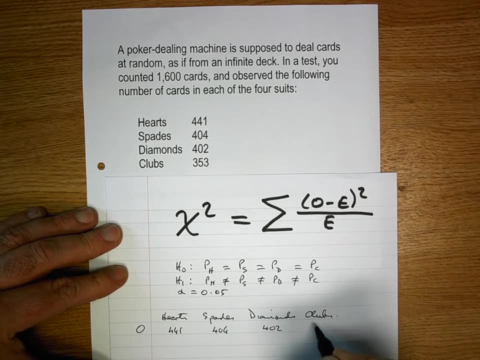 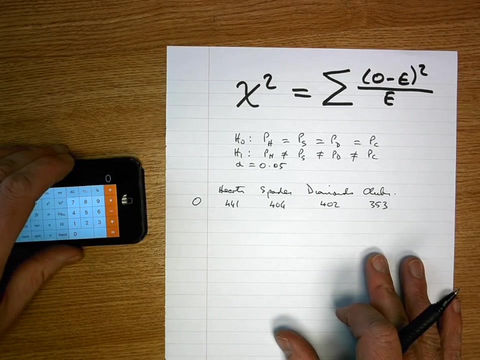 clubs And my observed values are simply the four values that I have up here. so I'm going to put in 441 hearts, 404 spades, 402 diamonds and 353 clubs, So I can take away my question there. now, give myself a bit of space. 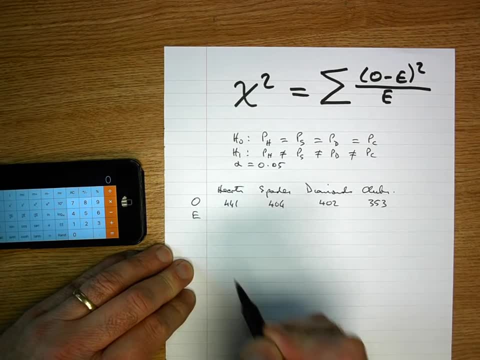 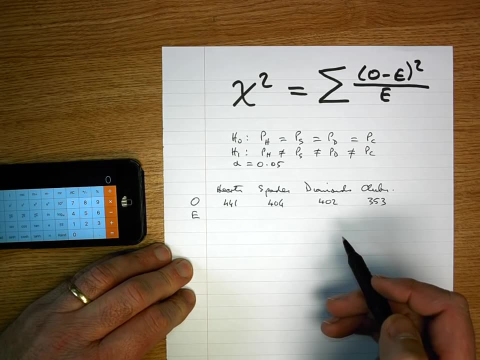 Next we have to put in our expected values. So that's going to be designated with an E And as we have four suits here and we have drawn 1,600 cards, we would expect each suit to occur 1,600 divided by 4.. 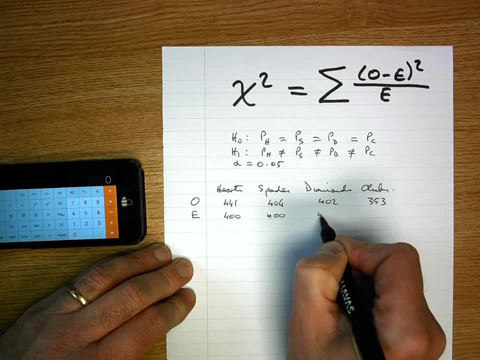 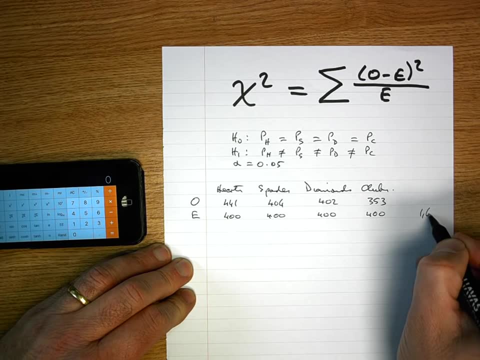 So we would expect exactly the same number of cards to be determined if they are drawn at random. So each of these two rows here adds up to 1,600.. So now we have the two values we need in our formula, so let's go ahead and work out the. 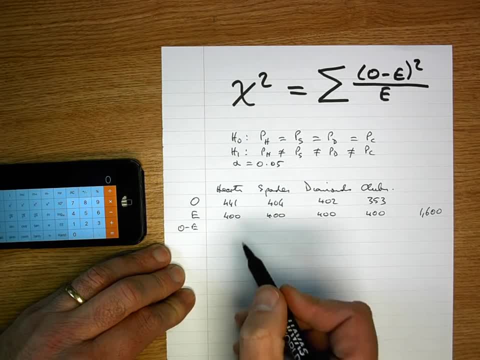 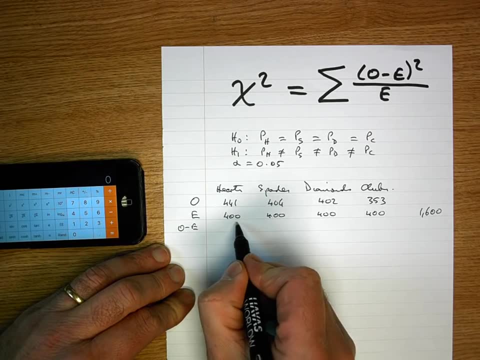 calculations. So first of all, let's do O minus E, and that's the difference between the observed and expected. You can do E minus O if you want. it doesn't matter which way you do it. So I'm going to do these first calculations in my head. 441 divided by 400, take away. 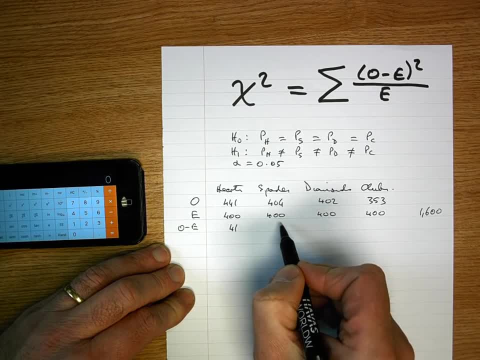 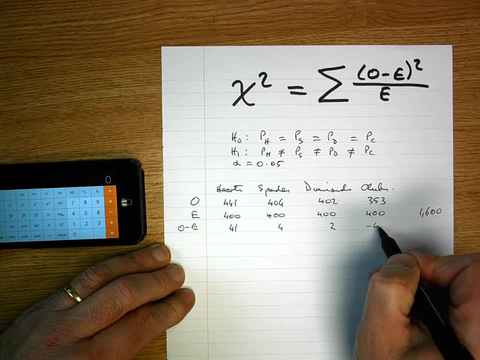 400 is 41,, 404 minus 400 is 4,, 402 minus 400 is 2, and 353 minus 400 is minus 47.. Next we can see in our formula that we need to square that value, so let's do O minus E. 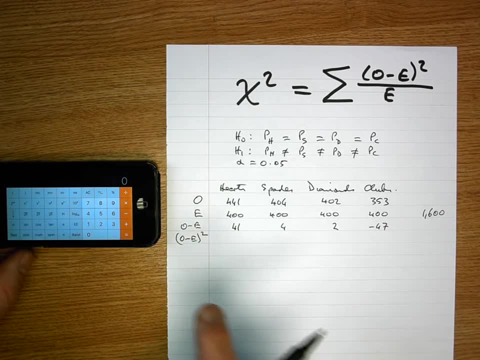 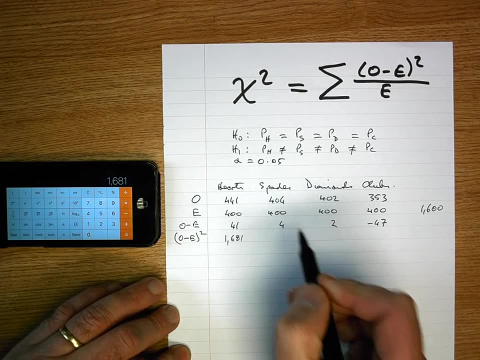 squared, so I need my calculator for that. So first of all, it's number: 41 squared that's 1,681, 4 squared in my head is 16,, 2 squared is 4, and minus 47 squared is: 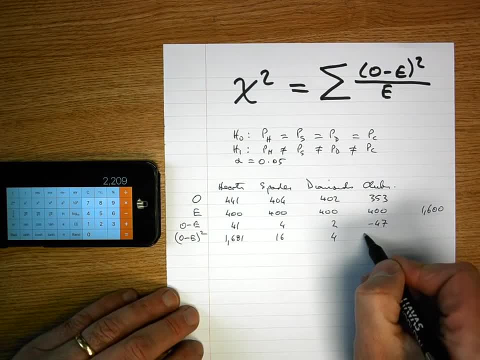 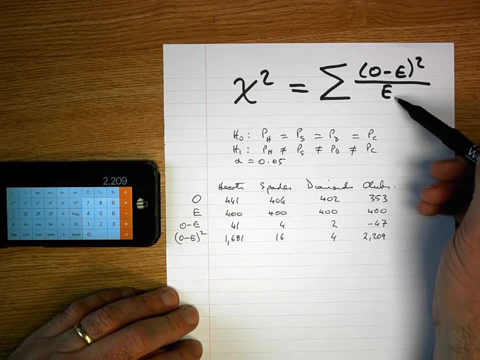 2,209.. The next part of the calculation is we need to divide that number by the expected value. so for hertz that's going to be 1,681 divided by 400, so let's write that in: O minus E. 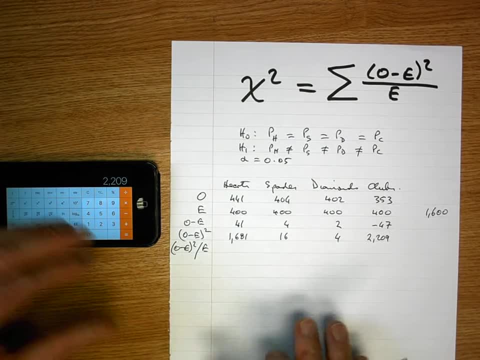 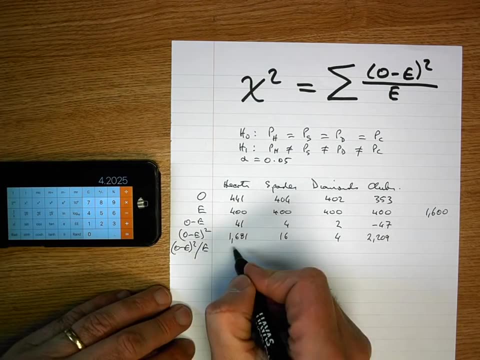 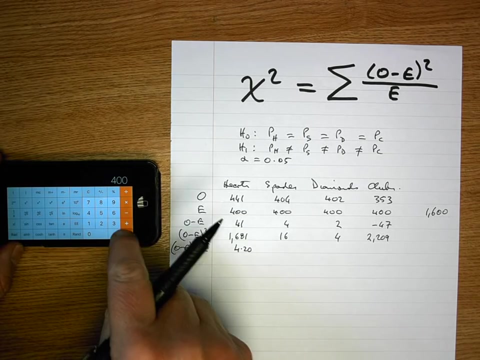 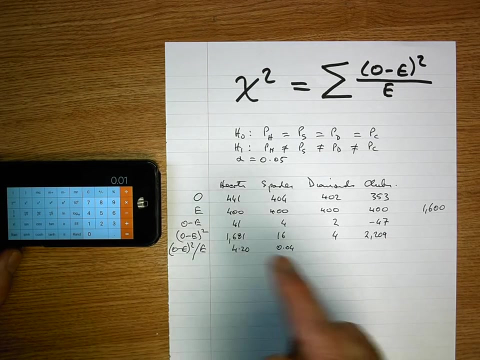 squared divided by E. so work my way through that: 1,681 divided by 400 is 4.2 rounded. Next is 16 divided by 400, that's equal to 0.04,. 4 divided by 400 is equal to 0.01, and the final calculation for clubs is 2,209 divided by 400,. 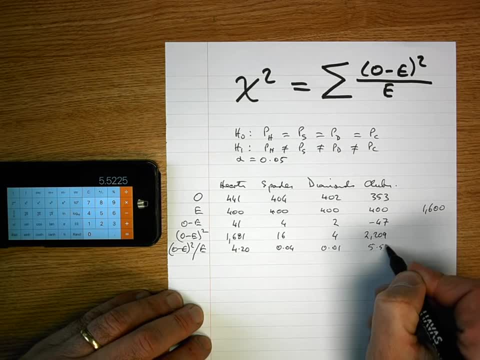 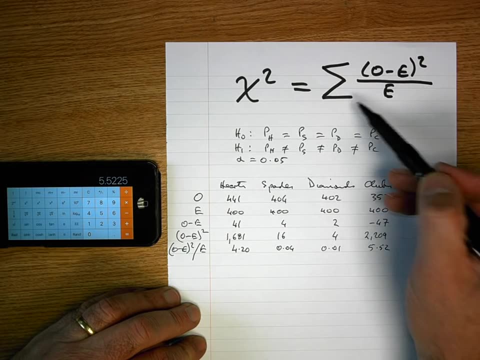 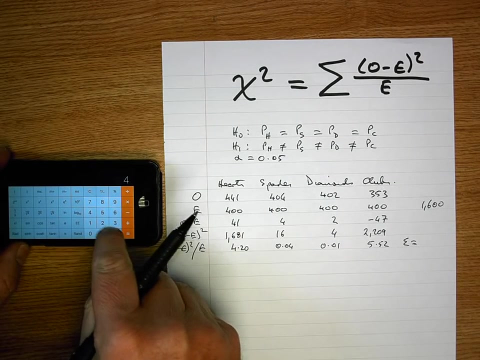 which is equal to 5.52 rounded. So we have four groups here. so we've now done this formula up here four times and now we need to sum them all together. So add these four numbers up. so let's go ahead and see what the sum of those four numbers is. So 4.2 plus 0.04 plus 0.01 plus. 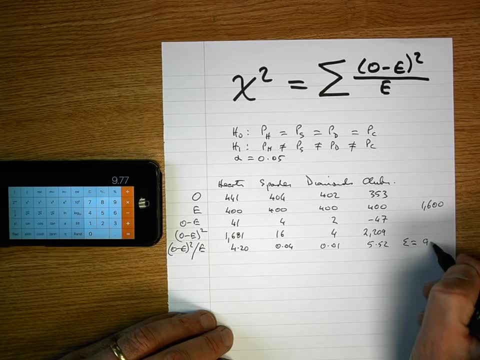 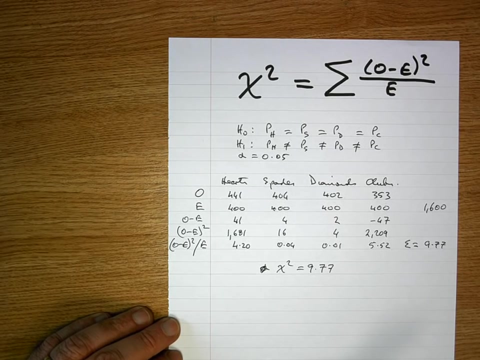 5.52 is equal to 9. 77. So my calculation here: my chi-squared value is equal to 9.77, so that's what we've worked out in this formula up here. Next, we need to determine a critical value from our chi-squared distribution. 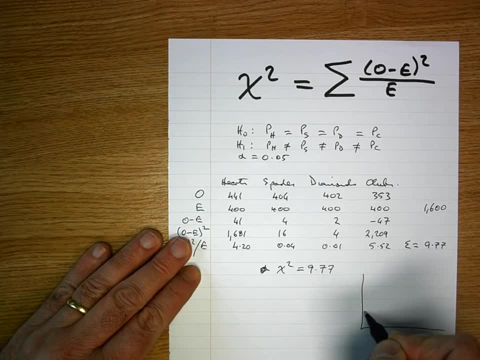 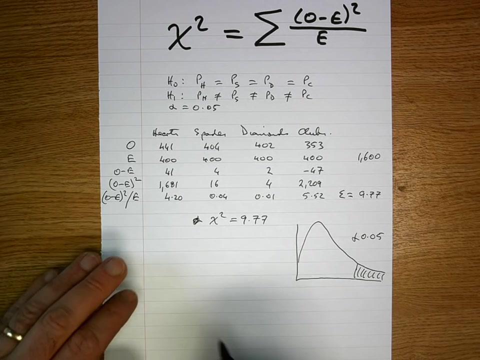 table. So we have a distribution something like this for chi-squared and in the right tail. we need to know what this critical value is going to be here at alpha, equal to 0.05.. So to do that, we need to determine first of all the degrees of freedom, so our degrees of freedom. 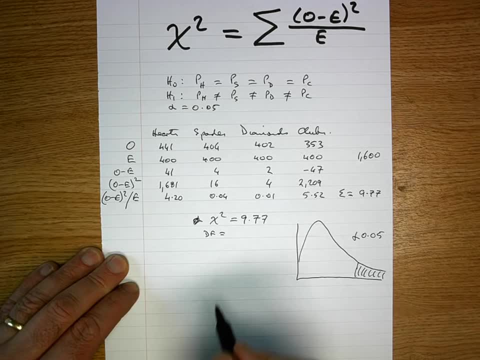 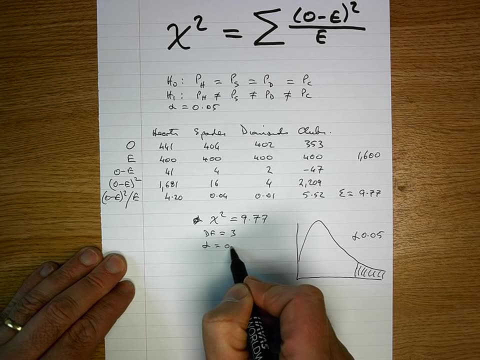 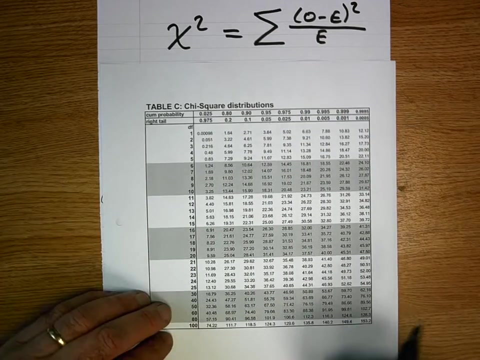 is going to be the number of groups minus one. so that's four minus one. so that gives me three, so three degrees of freedom. My alpha value: I already worked that out at 0.05, so I'm now ready to look up my chi-squared distribution table, which looks like this here. So I have right across. 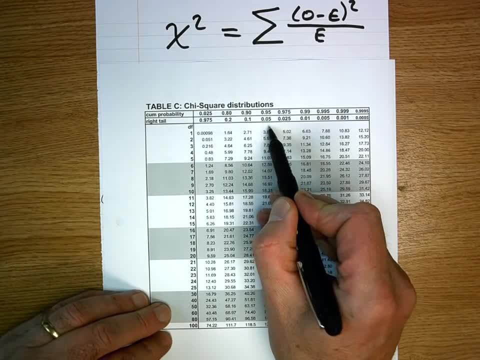 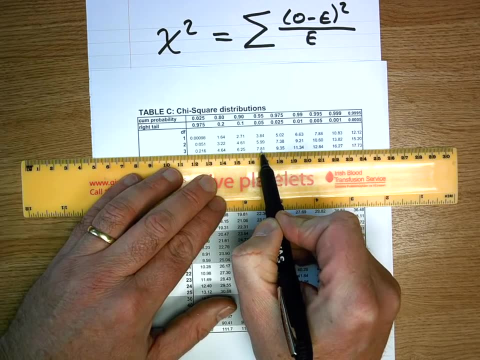 the top I can see what my probability is. so it's 0.05. I have chosen and the row I get it gives me three degrees of freedom. so where they intersect, a value of 7.81 occurs. so that's my critical value. 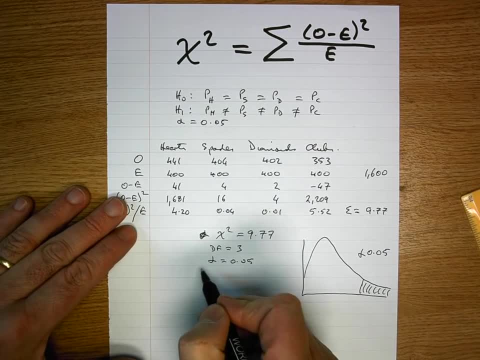 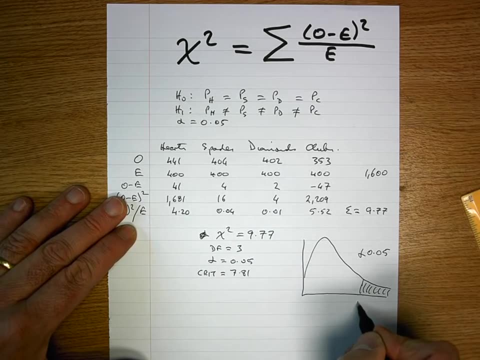 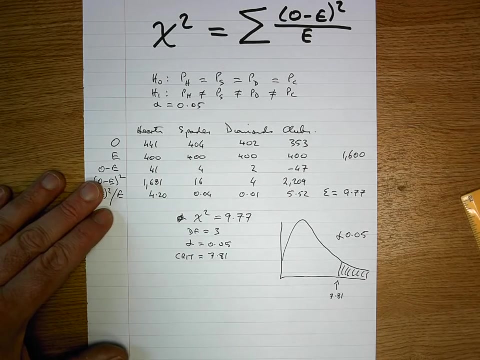 So my critical value is equal to 7.81, so here I can write in 7.81.. We can see that my chi-squared value exceeds that. so now it's time to report and make a decision. So we report like this: 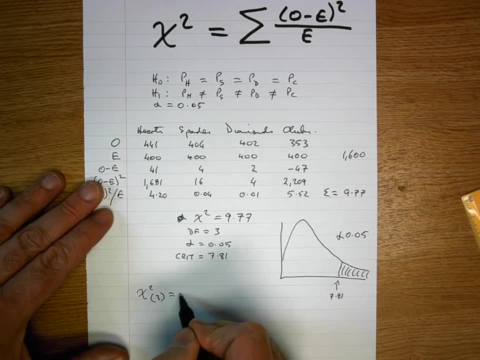 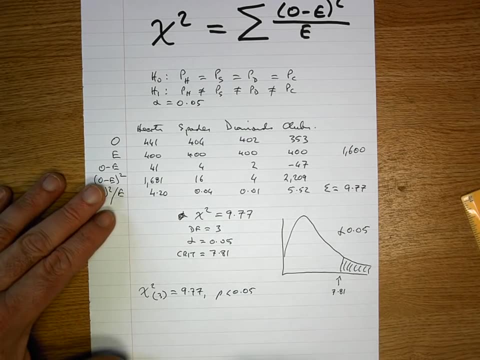 chi-squared for three degrees of freedom, it's equal to 9.77.. And our probability was set at 0.05, so that's how we report our result. We can see here that our chi-squared value is greater than our critical value, so our chi-squared value is going to fall. 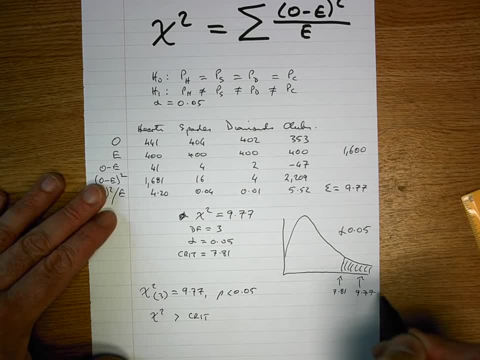 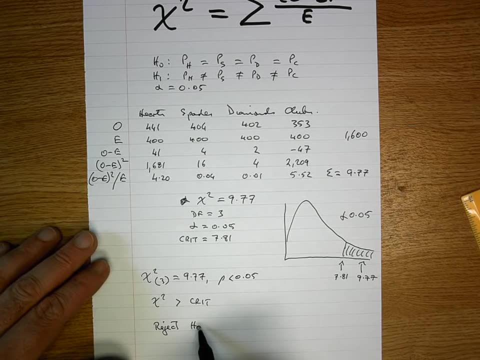 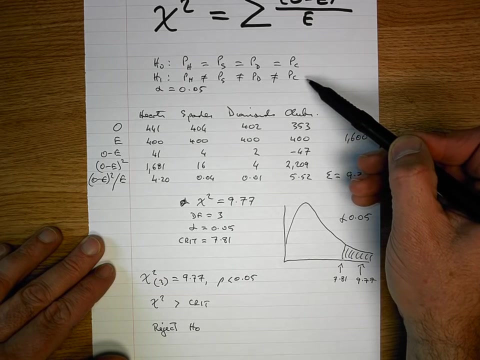 into the rejection region over here 9.77,. so therefore, our decision is that we reject our null hypothesis. So we're rejecting our null hypothesis that there's no difference between the observed and expected. in favor of the alternative hypothesis is that there is a 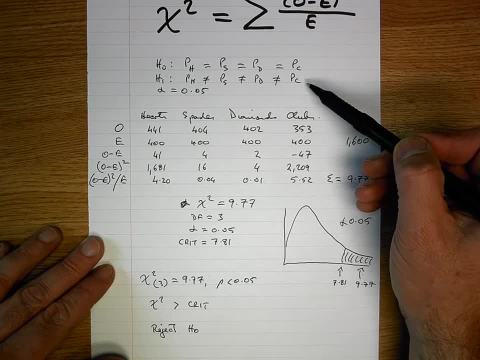 difference between the observed and expected. So we're rejecting our null hypothesis that there is a difference. So in this particular instance here we have found a difference and we might for example be concerned about the poker dealing machine that it's not dealing out cards at random. 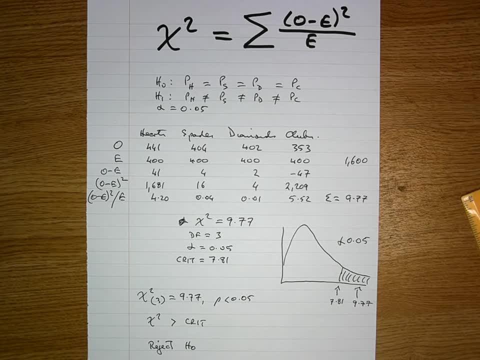 So that's how you conduct a chi-squared test by hand. I hope you found this video useful. Thank you for your attention.